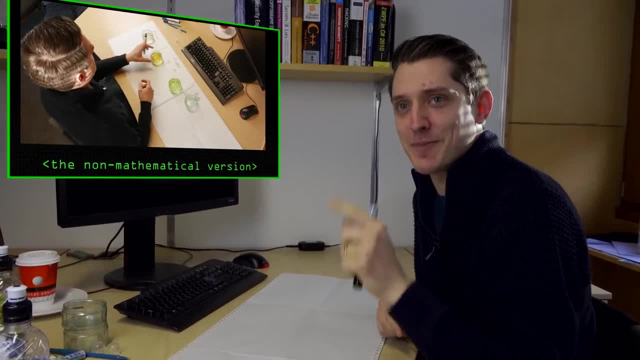 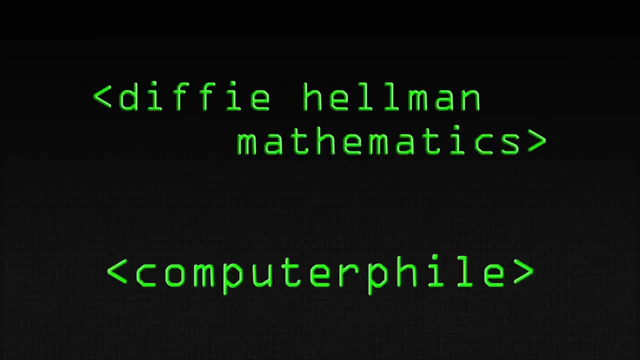 If you don't want to know that, there's a nice close button in the top corner or a back button. you know, be my guest, So that this is for mathematically inclined people. Let's go back to where we were before. So we have Alice and we've got Bob and we've got our public area here, sort of public. 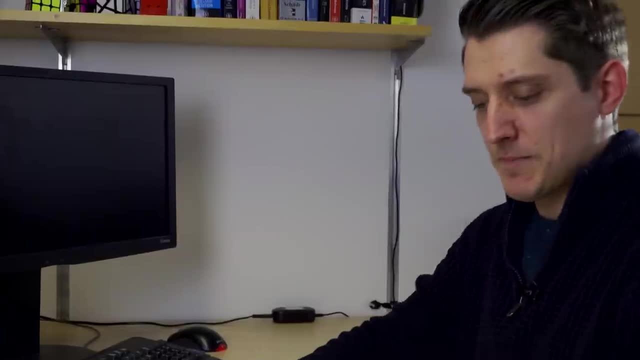 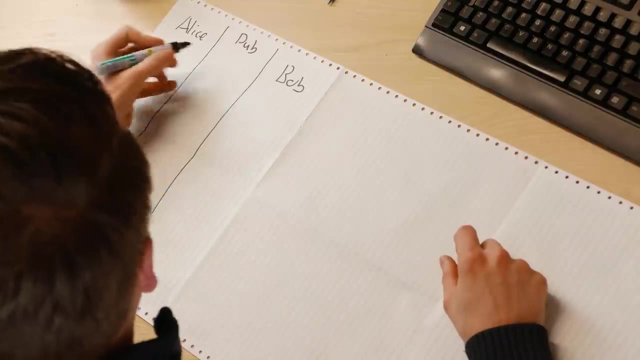 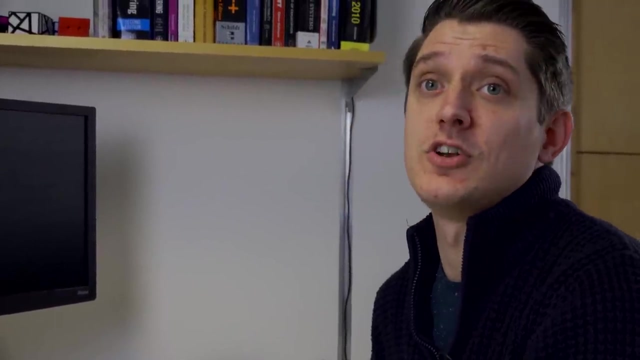 Public and we're going to draw down here Now the mathematics behind. Diffie-Hellman is usually modular arithmetic. Recall that we have our public numbers G and N. G is often very small. It's usually a small prime number. N is often very big and needs to be big for the security of this to work. 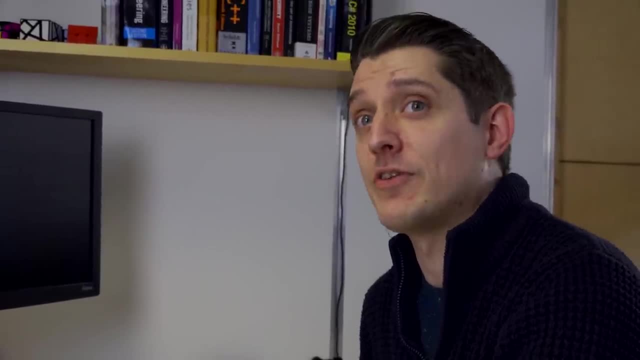 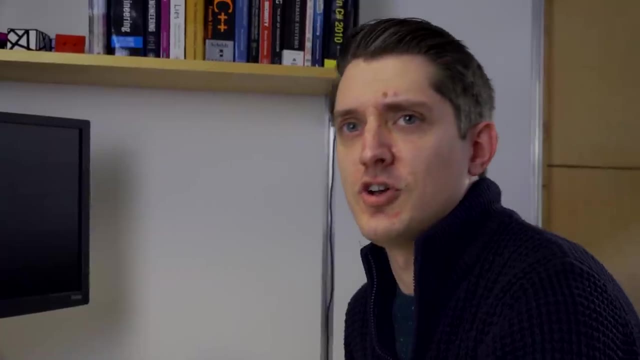 N is often 2,000 bits long, or 4,000 bits is more common now. So N is very, very big. It can't be too big because you won't gain much in security that you lose in efficiency. So you know you have to think about that. Alice and Bob need to pick their numbers A and B. 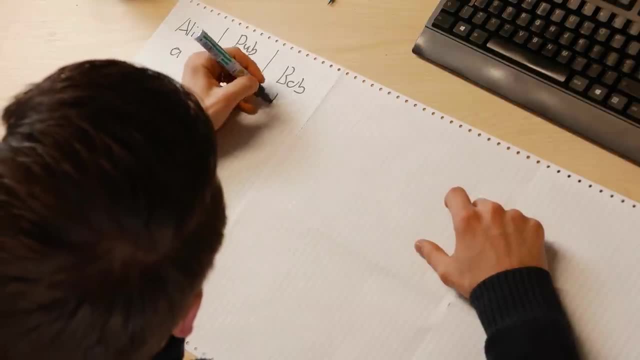 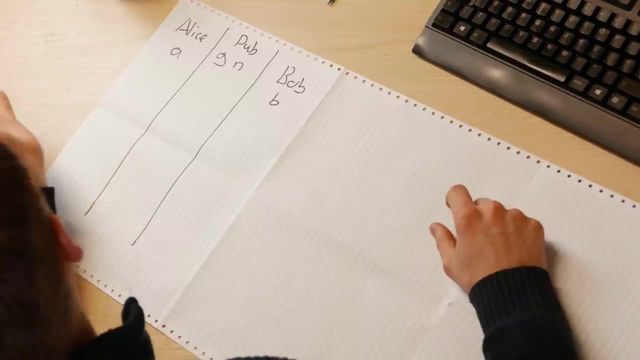 So Alice picks a number A, Bob picks a number B. These are the ones they're going to keep private. Now, A is somewhere between 1 and N, but it's random and N is so vast that it's not going to be 1.. 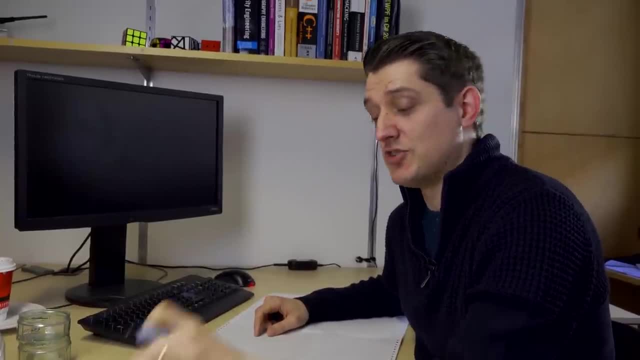 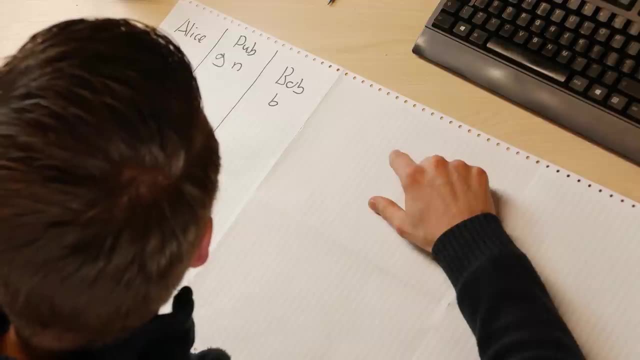 It's going to be a very big number. Let's not worry about what it is. She's not going to tell anyone what that is. Same for Bob. The first thing Alice does is she calculates G to the power of A mod N. 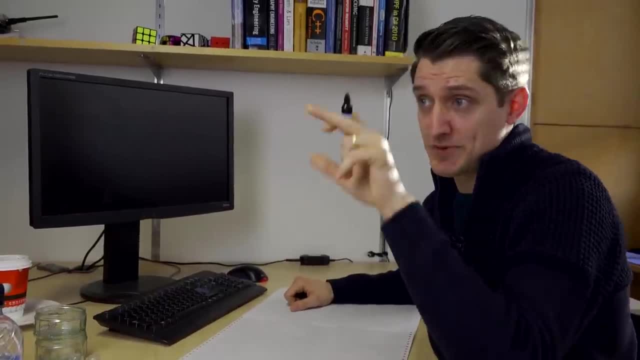 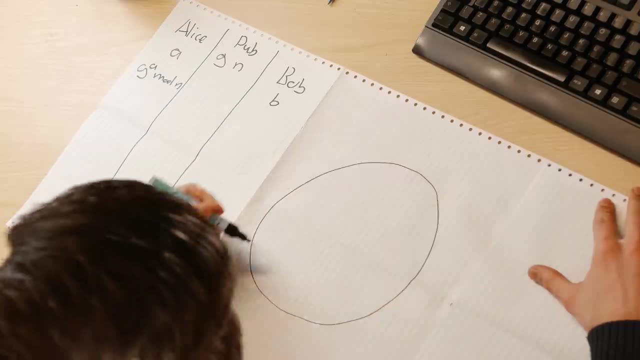 Right Now, modulo, if you do any programming you'll be familiar with the percent symbol- is the remainder after division. So another way of looking at modulo is to have this kind of clock face. So if we have a clock face, which should be a circle, and we go from 1,, 2,, 3, all the way round to N, 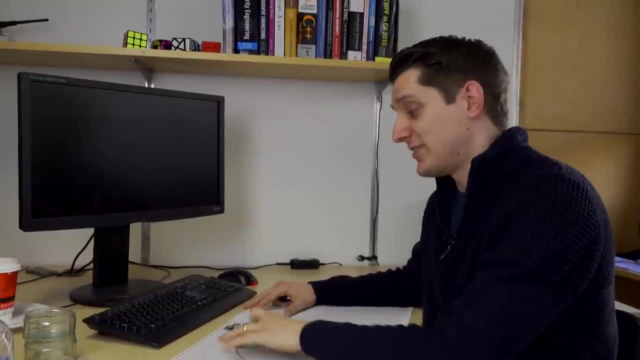 These are the numbers modulo N. So when we perform some arithmetic in this space, we just go round and round the clock face. We don't ever leave and go above N or below 0. In fact, this should be 0 as well. 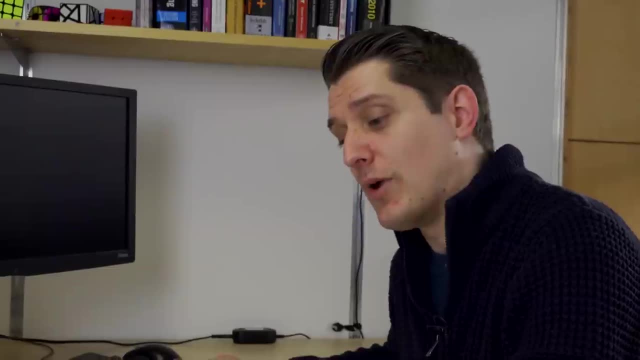 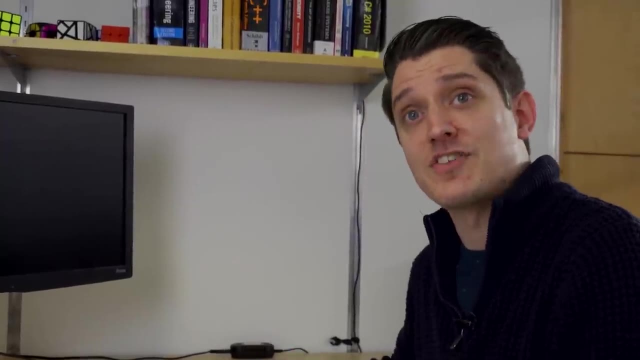 There should be a 0 in here. So when you do G to the power of A mod N, what happens is you're raising G to the power of some massive number, which would be very normally very big, But in actual fact it just goes round and round this clock face and ends up somewhere. 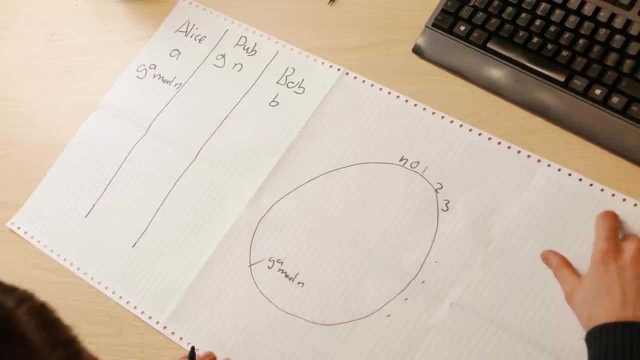 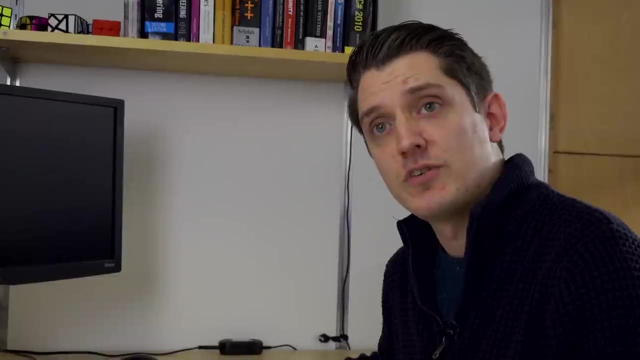 So let's say G to the A mod, N arrives somewhere here on the clock face. Now, what's important about this is: it's very difficult, given this, to work out what A was. We know G is, let's say, 3, right, If I say we're here on the clock face and we started at 3,? 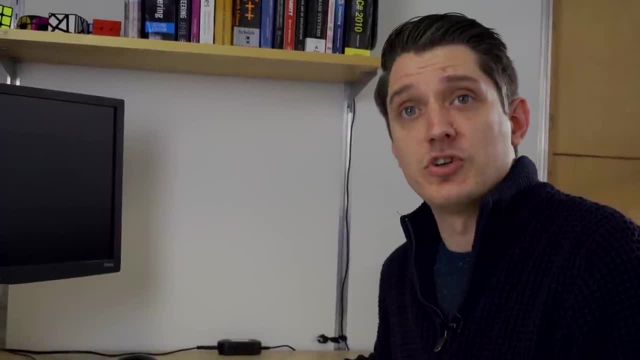 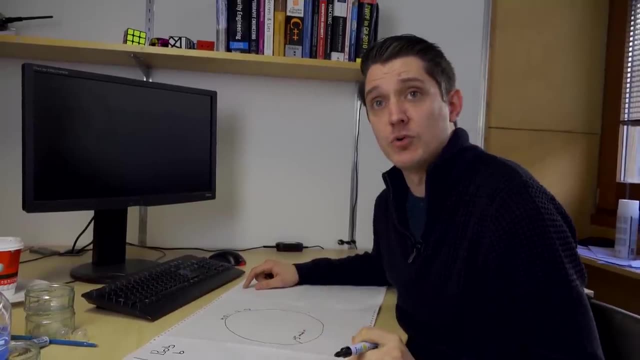 what number is A? It's just impossible to know right, Because its position on this clock has no bearing on how many times it's gone round or what A was at all right. The only way to do this is essentially to brute-force it to go well. is it A to the power of 1?? 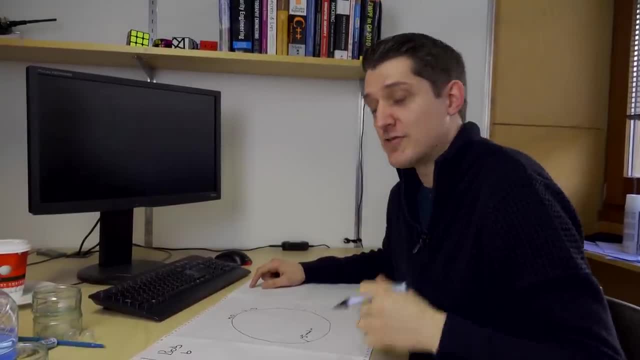 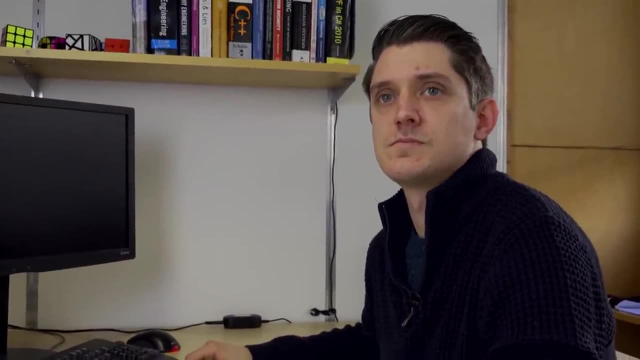 No, it's not. Is it A to the power of 2? No, And then so on and so forth for an infeasible amount of time. We did a little bit of this with the hashing video, didn't we? There was a little bit of the modulo function there in calculating the hash. 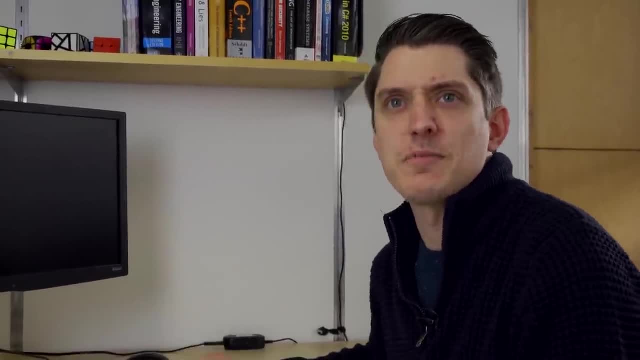 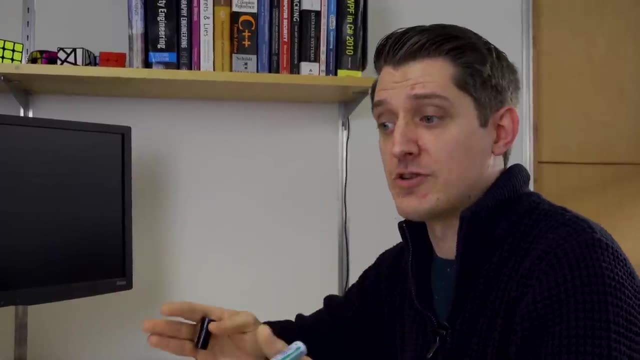 Yeah, so that was used to shorten something at the end, But it's the same kind of principle. Modulo is very useful for taking something that could be any length and putting it into a sort of finite loop, a finite group of actual numbers. 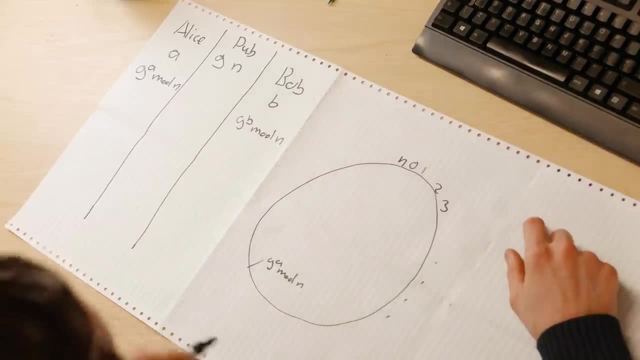 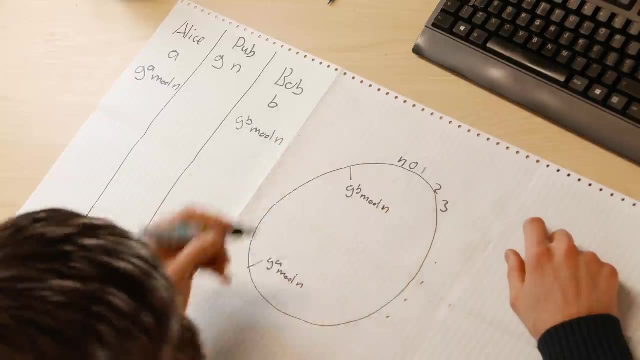 Now, Bob, we're going to take G to the B mod N. So let's say, that turns up over here somewhere. So this is G to the B mod N. So again, what we've done is we've taken G, we've raised it to the power of B and we've done all of this. modulo N. 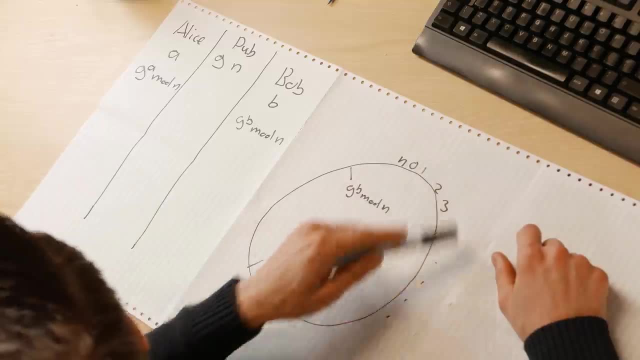 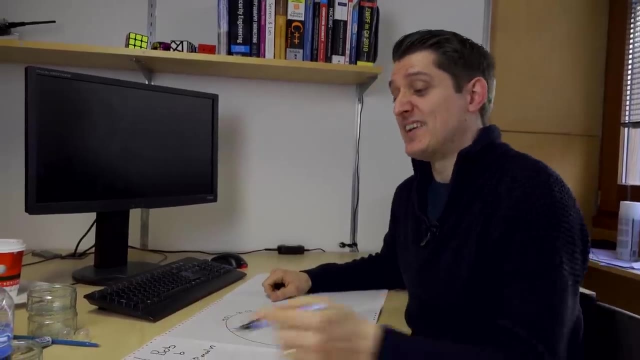 which means that it just if it ever goes above N, it just loops back down to 0 and keeps going. So this is somewhere else. These are their two public components, So they share these like this. So now these are public. But again, calculating A and B from this is very, very difficult. 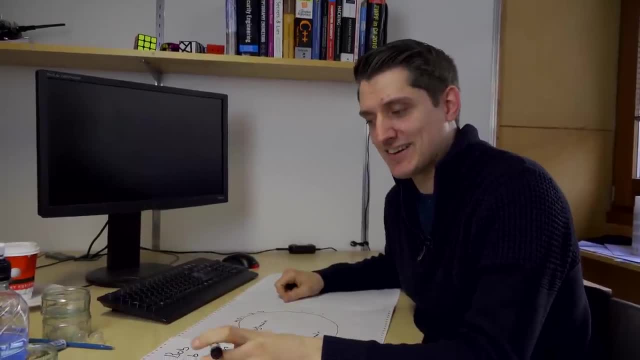 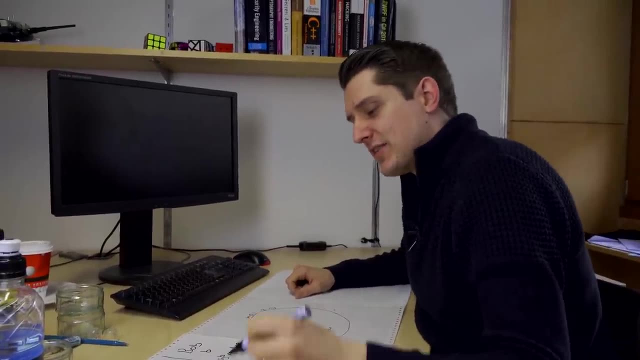 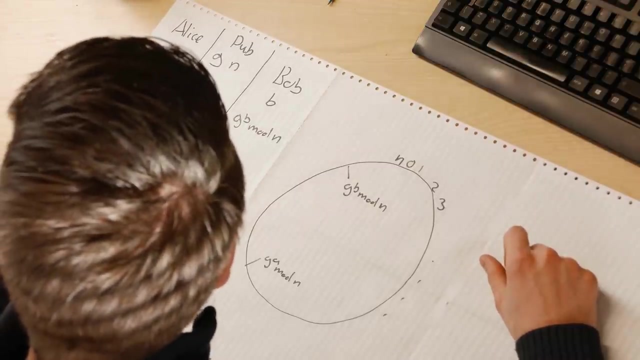 It's called solving the discrete log problem and practically very, very difficult for even a supercomputer. Now Alice is going to take this. I'm just going to simplify the notation slightly to make it fit on the page. But Alice is going to take the G to the B that Bob sent and raise it again to the power of A mod N. 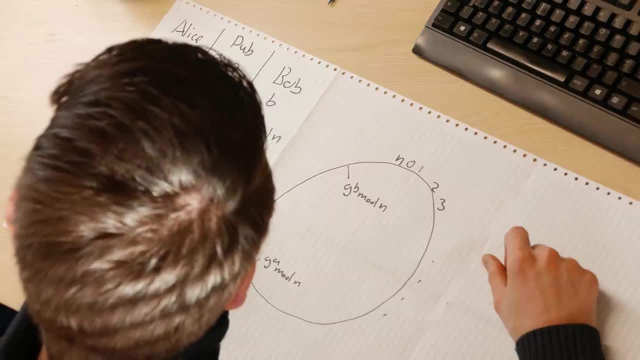 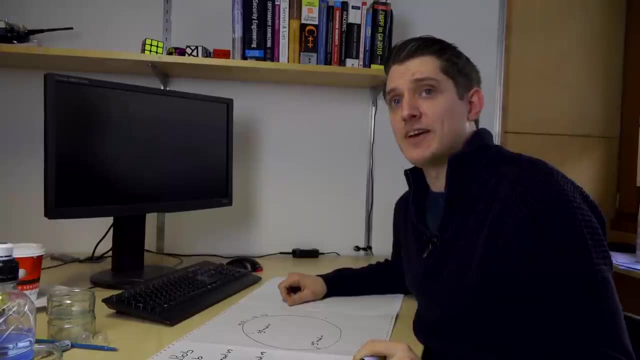 And Bob is going to take G to the A that Alice sent and raise it to the power of B mod N, And anyone that's done any exponentiation knows that if you do something to the power of something, to the power of something else, it's actually just those two things multiplied. 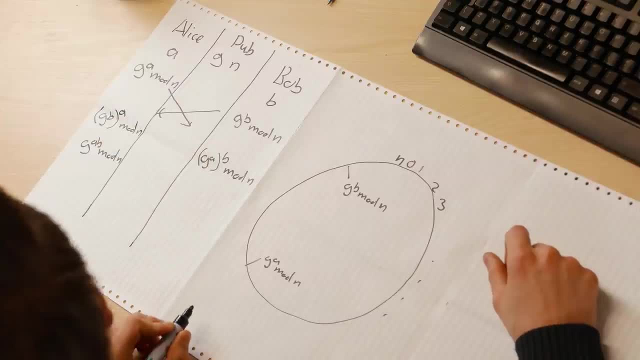 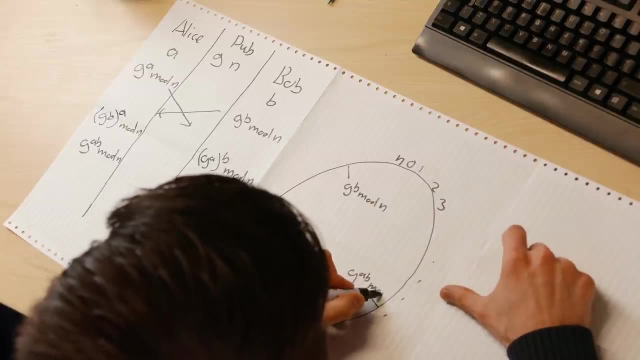 So it's G to the A B mod N. That's the answer. So that will come somewhere around, you know, let's say here: So this is G to the A B mod N. Now this will be some number between 0 and N. 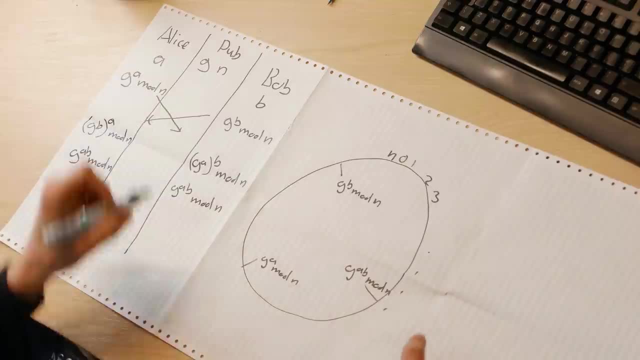 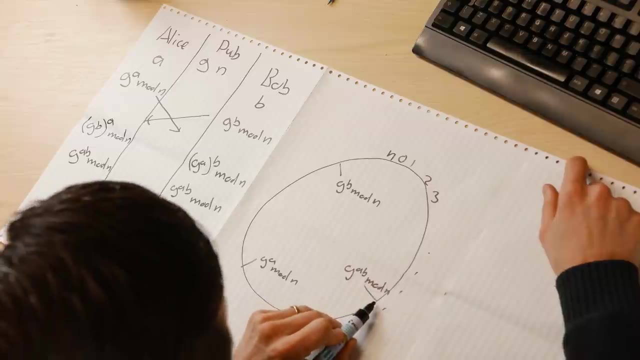 Bob's done the same thing. He's also got G to the A B mod N, And They're exactly the same. These are two identical colors we were looking at in our color example, So they've both arrived at the exact same position in this group. 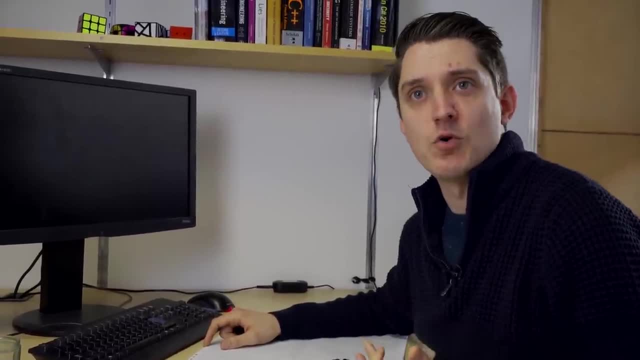 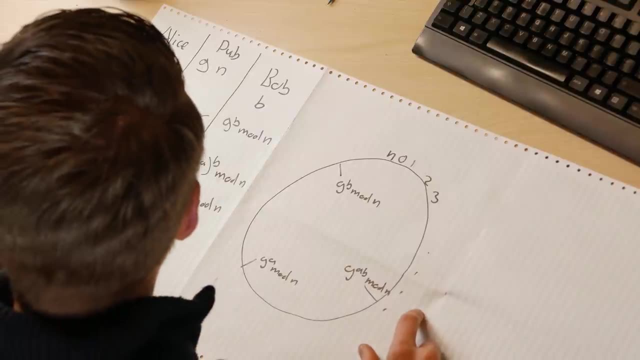 despite the fact that neither of them knew what each other's private key was. That's what's really cool about Diffie-Hellman. To try and reverse this process, we have to know A or B. We know- publicly- G to the A. 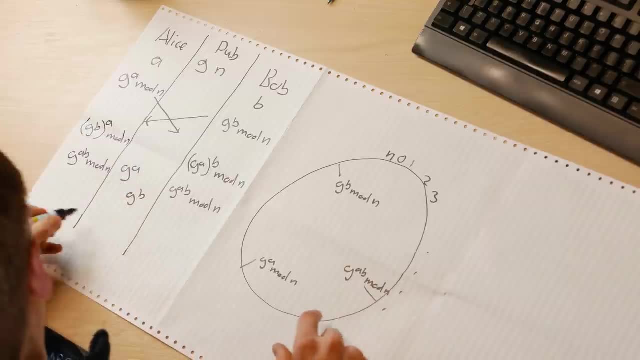 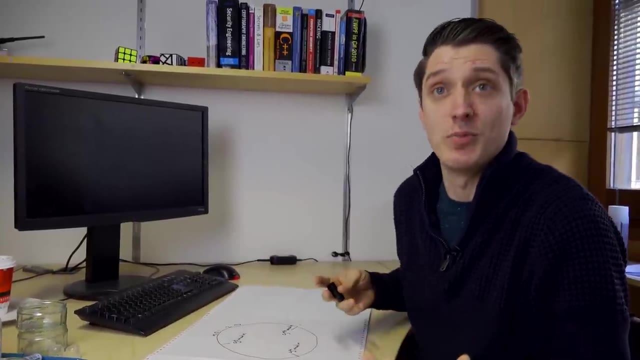 And we also know G to the B. If we try and multiply them together, for example, we'll get G to the A plus B, which is not the same Right. that's me sort of mixing my public colors together in the hope of getting the right answer. 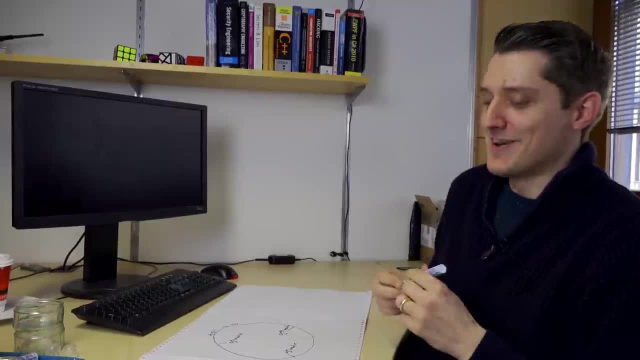 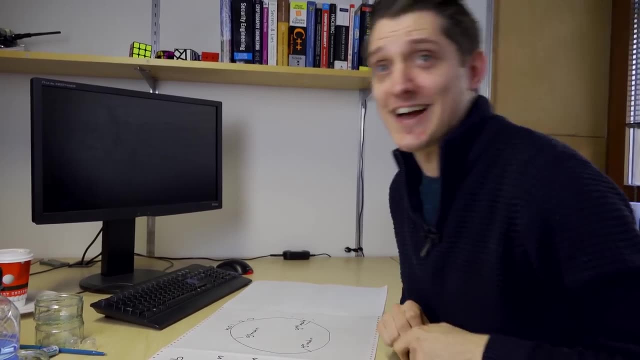 I haven't got it. That would be somewhere else, a completely different number. Remember, this is cryptography: If you're one position out, it's not going to decrypt, right? So you know you have to get it exactly right. 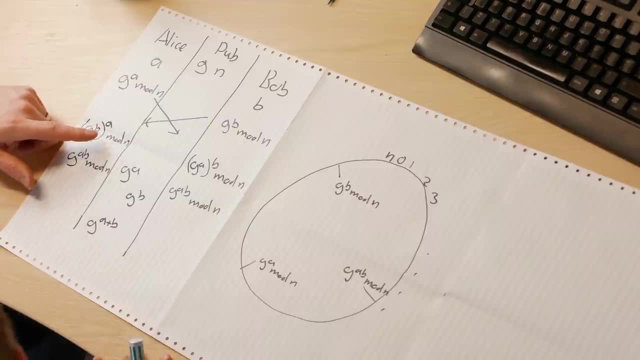 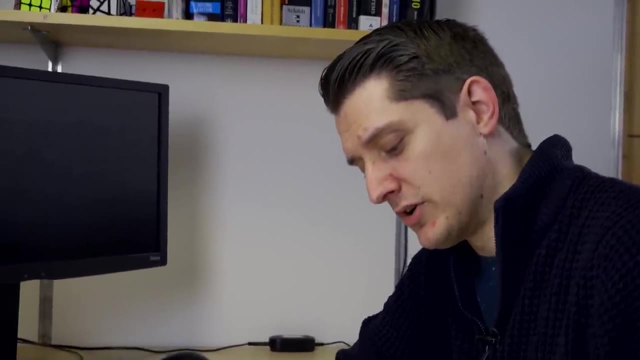 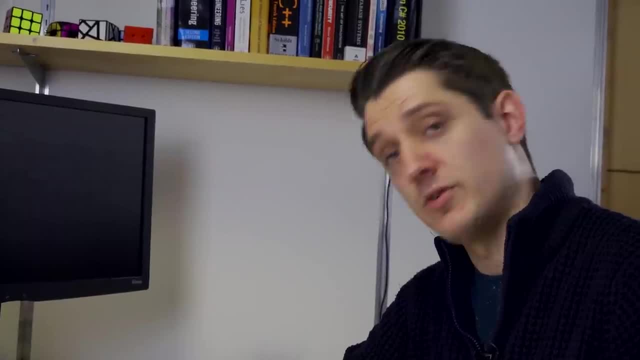 That's 2 times 2 times 2 times 2 to the power of 3.. That's 2 times 2 times 2 to the power of 3.. That's 2 times 2 times 2 times 2 to the power of 3, right. 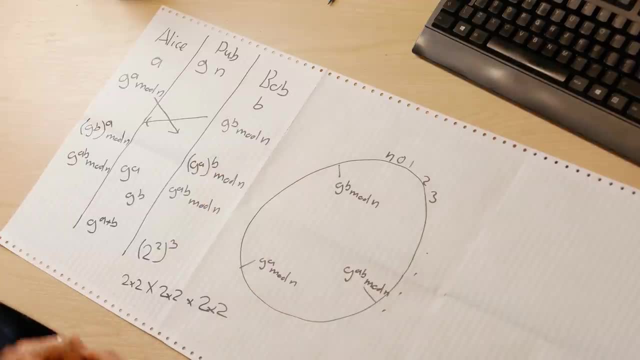 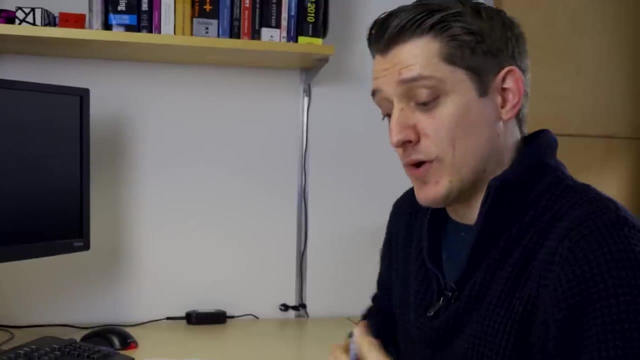 Which is 2 to the 6, because there's 6 of them. You can do it in any order, It doesn't matter. You get the same number out at the end, whereas that is a completely different thing. Yeah, so that is equivalent of. 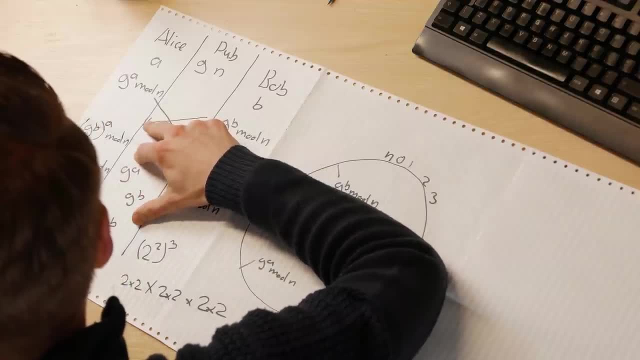 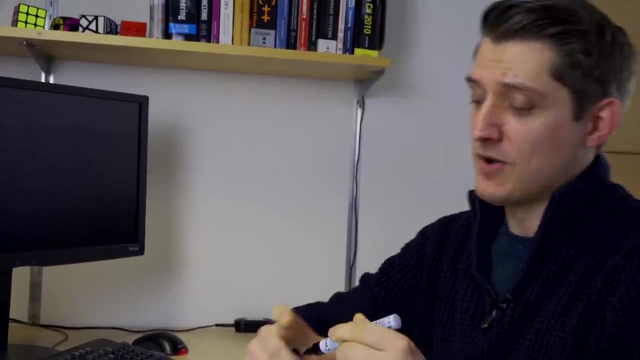 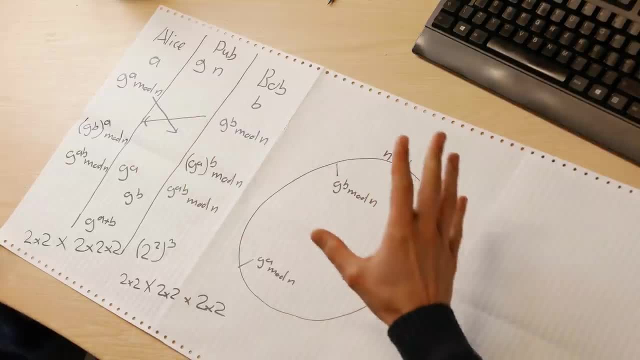 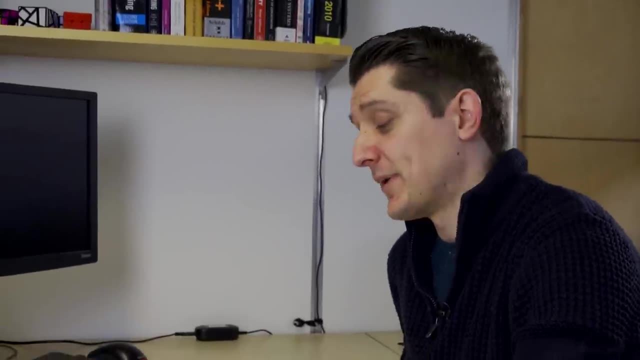 Going to be somewhere else completely on this, on this modular arithmetic clock, face You're not going to. it's not going to work at all. the n number is kind of important, though, Is it right? It's mostly important that n is big, because if n is small, then